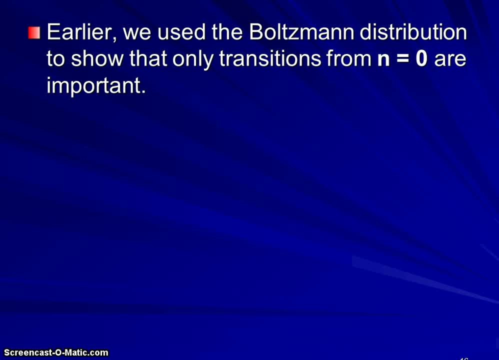 distribution to show that for vibrational transitions, only transitions that go from n equals zero to n are significant, Because most at room temperature the molecules will be in the n equals zero energy level. So we substitute the spherical harmonics from chapter 7 and the expanded dipole moment in 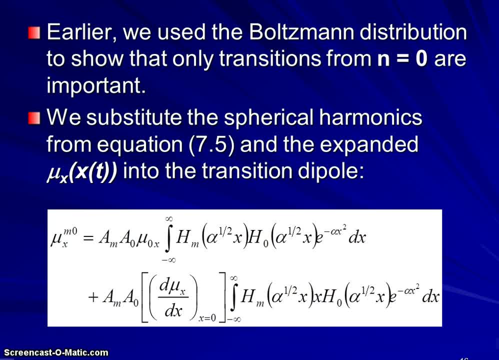 for the transition dipole. And look what we have here. These are the normalization constants for the spherical harmonics. The permanent dipole is a constant, So that can be pulled out in front. And then so we have the spherical harmonic for a particular energy level, the spherical 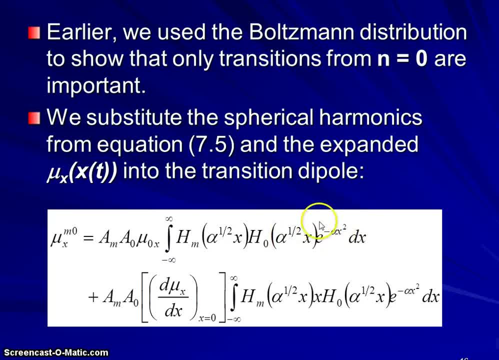 harmonic for the zero energy level, the rest of the wave function, And then here we have the transition dipole, also a constant pulled out in front, And then the spherical harmonics. Now the transition dipole in our previous equation was multiplied by x. 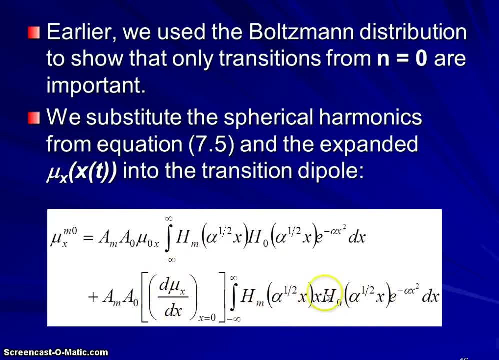 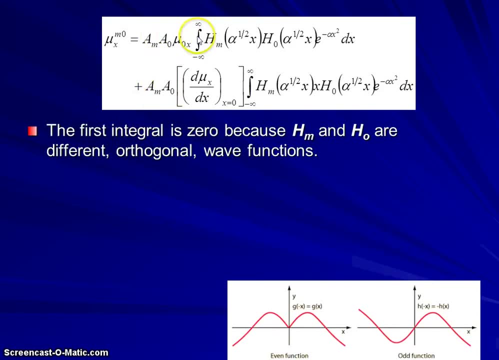 So we have x here and then the rest of the function. Now I want to bring that equation over to the next slide so that we can talk about it a little bit. This first integral is going to be zero, because these spherical harmonics are different: orthogonal. 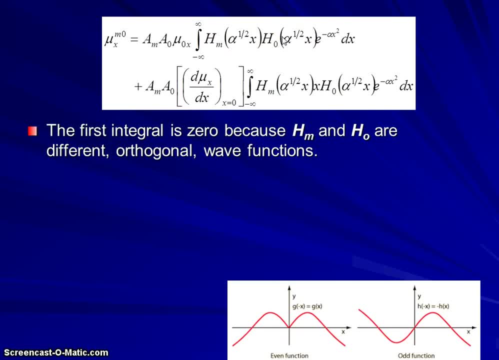 wave functions. So in order to multiply When we multiply, we multiply, When we multiply them by one another and take the integral, then we will see zero here. Now, the second term will be integral, I'm sorry, will be zero if the entire integrand is an odd function. 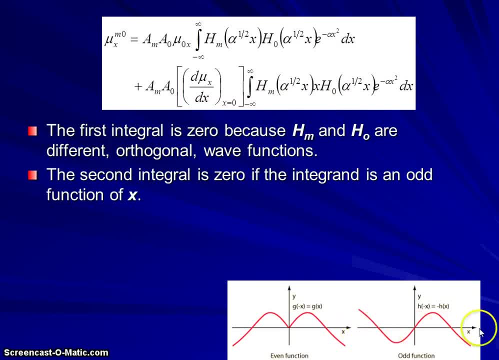 Think about the area under the curve. If we're working from here to here is going to be on this side. the negative of this side will add up to zero. So Let's think about what that means, since the zero energy level harmonic is an even. 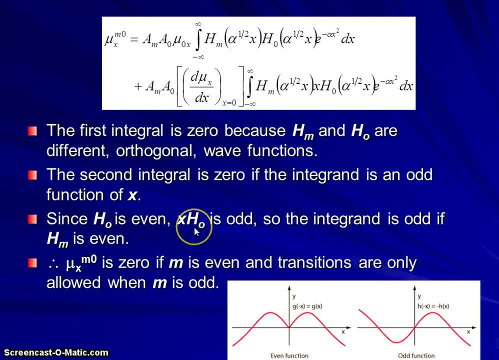 function X times, that will be an odd function, because an even function times an odd function is odd, So the integrand will be odd if the transition level that we're going to is even. Therefore this function, the transition dipole, will be zero if m is an even function. 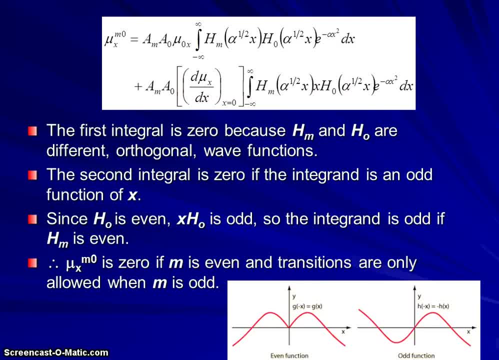 And so transitions are only allowed to energy levels where m is odd, so that we get a nonzero sum under the curve, a nonzero integral. So our most common and most visible transition, The visible transitions, are going to be those that are from n equals zero to n equals one. 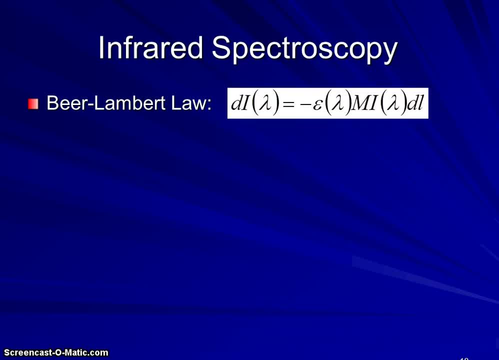 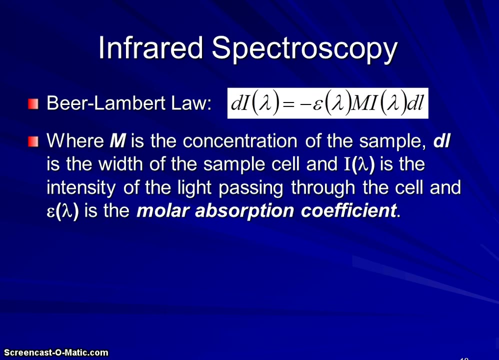 Let's think about this in terms of infrared spectroscopy. The Beer's-Lambert law relates the change in intensity of a particular wavelength of light as it passes through a sample to the concentration of that sample. So In this equation I've listed here, dL is the width of the sample cell we like to set that. 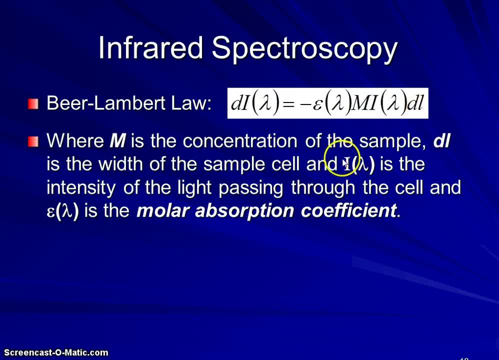 to be one centimeter. Intensity is the intensity of the light that we're passing through the electromagnetic radiation Epsilon at a particular wavelength is the molar absorption coefficient how much light that molecule absorbs per mole. And so this is the change in intensity. 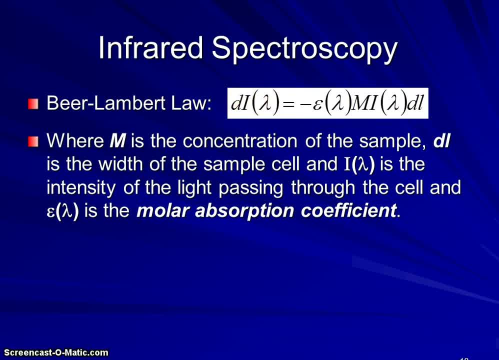 The difference in intensity that we find on the other side of the cell at our detector. If we integrate that equation we get that the fraction of the intensity that makes it through to the detector compared to the original intensity is e to the negative molar absorptivity. 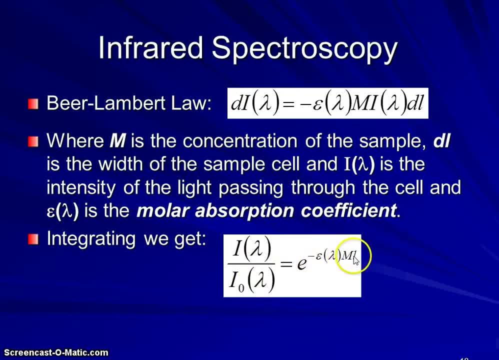 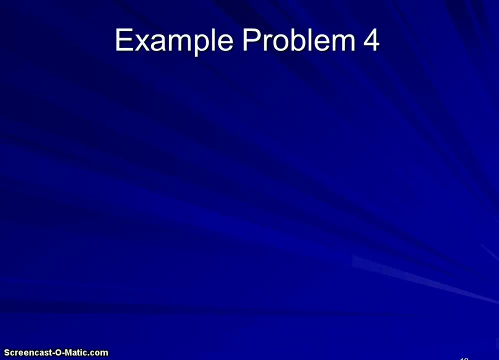 coefficient times, concentration times, cell length, So So So in this case, we can use this to get the wave length, And remembering that the molecular absorptivity coefficient depends on the wavelength. Now so take a moment to pause the video and write this problem down. 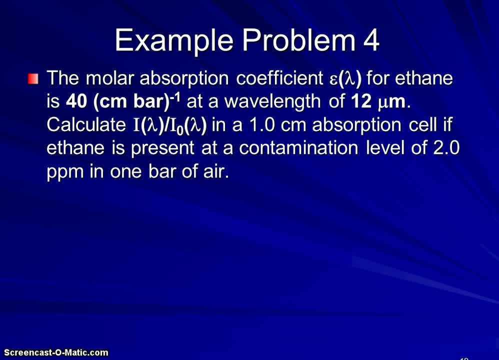 This is one that we'll work together on next time in class. I'd like you guys to give it a shot. based on the Beer's-Lambert law, The molar absorption coefficient for ethane is 40 reciprocal centimeter bars at a wavelength. 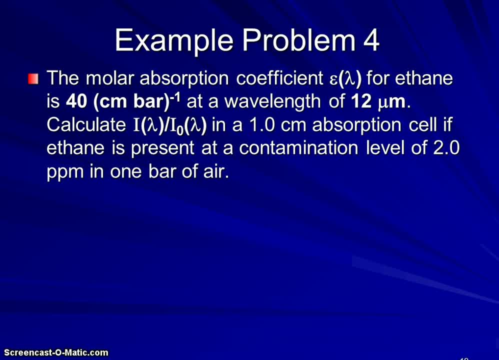 of 12 microseconds micrometers calculate that fraction in a one centimeter absorption cell if ethane is present at the normal contamination level of two parts per million, and then talk to us about whether it would be practical to try to detect ethane in a cell that size at. 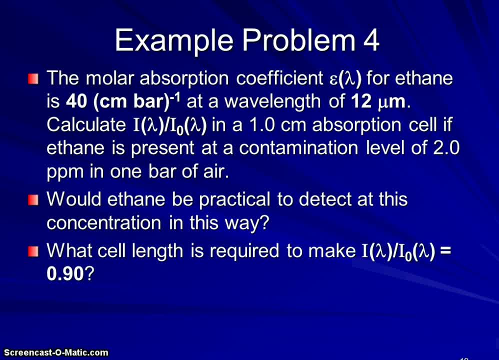 that concentration, Then calculate how big a cell would be required at two parts per million to get a 90% absorption, a .9,, I'm sorry, a 90% transmission, .9 transmission fraction. And then think about it, that's going to be a fairly long cell length. I'll 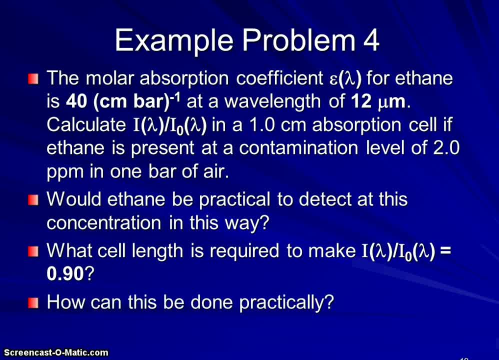 let you calculate it out. So the question is: how can we detect ethane at the parts per million level? if we want to use one centimeter cells- And I'll give you a hint- it can be done. but we'll work that all out in class. Try it on your own, please, sometime in the next day or two. Now. 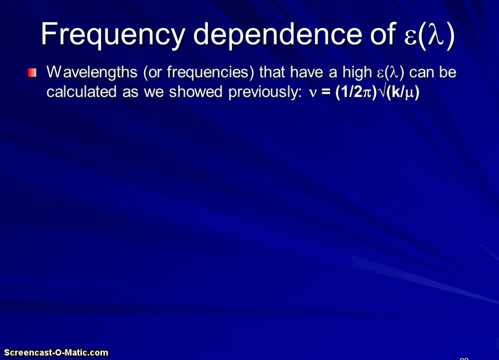 as I mentioned earlier, the molar absorptivity coefficient does depend on frequency and certain molecules will have wavering frequencies. Now this is true for all molecules. There are many molecules that have wavelengths or frequencies that have a very high molar absorptivity constant, and we can calculate what those 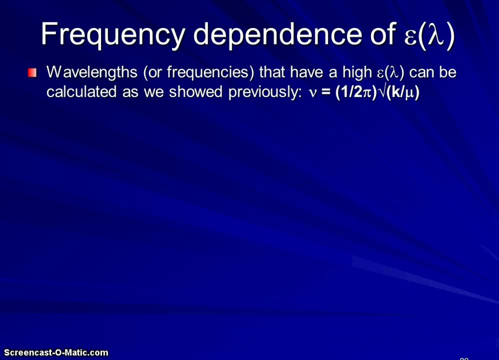 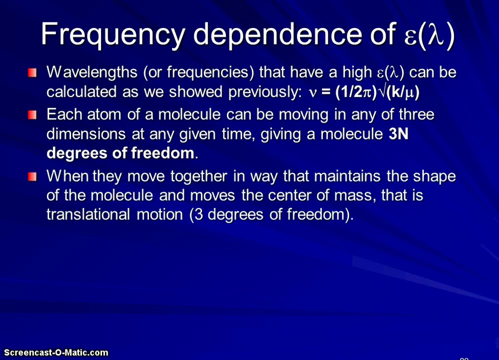 frequencies will be based on our quantum mechanics results from the previous chapter. Each atom of a molecule can be moving in any of three dimensions at any given time. that gives that molecule 3 n degrees of freedom If they move together in a way that maintains the shape. 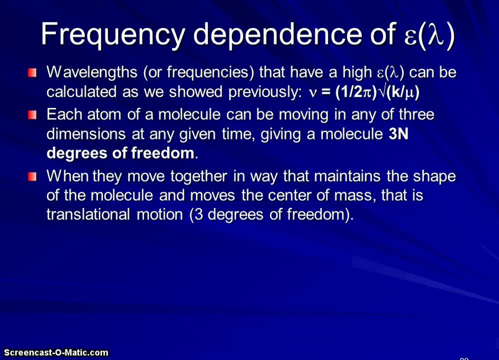 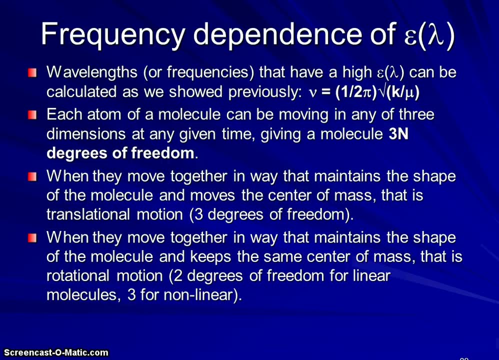 shape of the molecule and moves the center of mass. we call that translational motion. so that uses up three of the 3n degrees of freedom, where 3n is three times the number of atoms on the molecule. if they move together in a way that maintains the shape but keeps the center of mass the same, 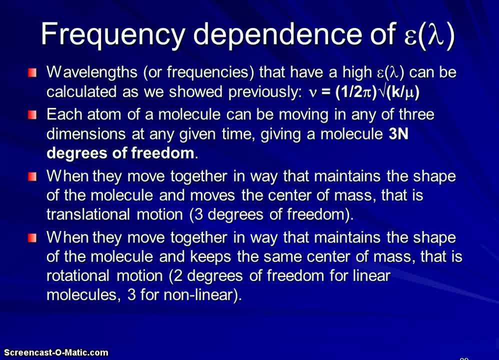 in the same position. that's called rotational motion, and for linear molecules there are two degrees of freedom. used up that way, there are two ways. linear molecules can rotate and non-linear molecules could rotate in three different dimensions. so the number of vibrational modes we expect to find is 3n minus 5 for linear molecules and 3n minus 6 for non-linear molecules. 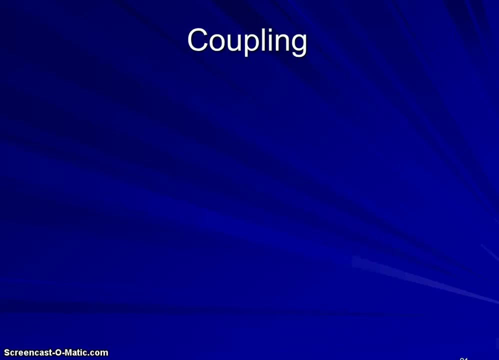 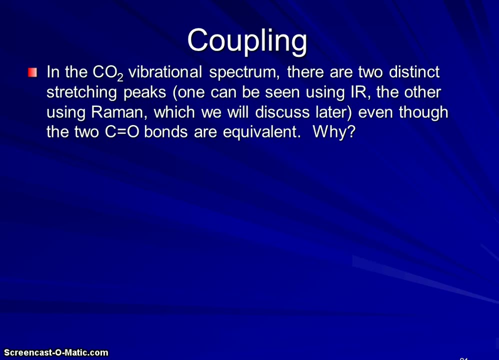 now let's talk about that in a fairly small molecule case. talk about a phenomenon we call the 3n-molecule case, and we'll talk about that in a fairly small molecule case. coupling CO2 is a linear molecule with three atoms, so 3n would be 9. since it's linear, we'll 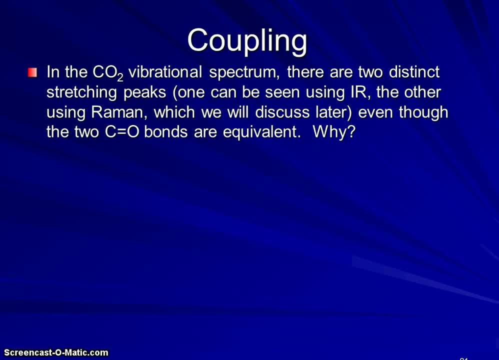 look at 3n minus 5, that gives us four vibrational modes and I want to talk about a couple of those vibrational modes, because we see CO2 as having two equivalent CO bonds, but there are two stretching peaks associated with those CO bonds. one of them can be seen in the infrared and the 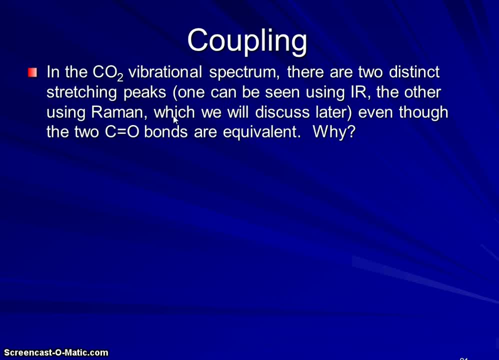 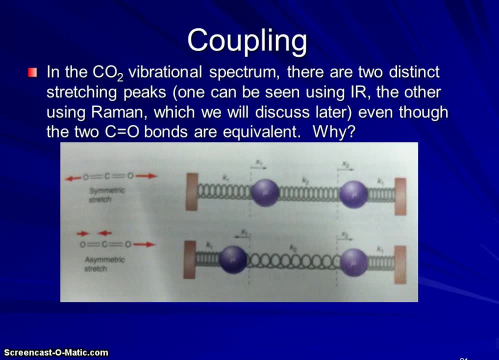 other can only be seen in the Raman. it does not meet the infrared selection rules. now let's talk about, then, the way that we think of CO2. when one C double bond O vibrates, the atomic positions and electron distribution throughout the molecule are changed. that would influence the 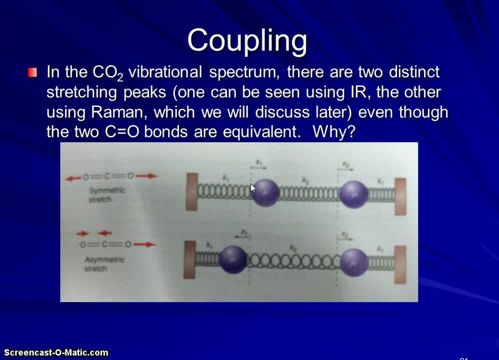 other CO bond. so they don't vibrate independently, since they are the same bond strength and one is influencing the other one they're going to violate. they're going to vibrate in conjunction with one another. they are coupled harmonic oscillators, and we can see what we mean here in this diagram. 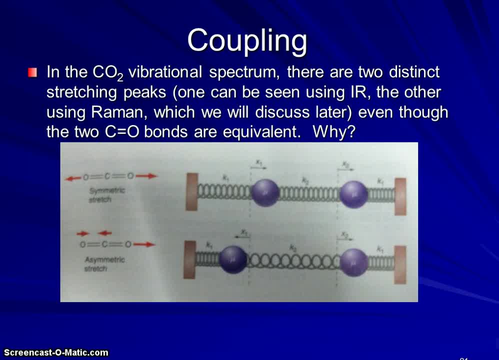 so what we'll do is think of each of the two CO groups as a mass coupled to a wall by a spring with force constant k1. so this is representing a CO bond. this is representing a CO bond and we modeled a couple as the coupling, the couple of them as a second spring with force constant k2. that 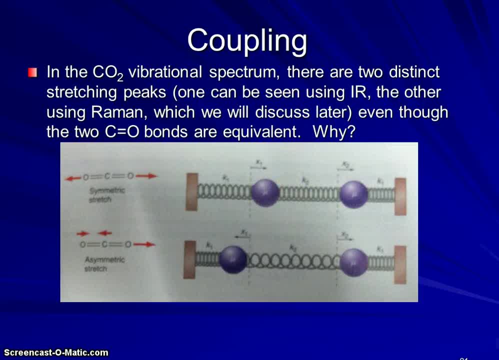 connects the two oscillators. if we assume that for the symmetric case, this is the third and follower of the TL, which has the same friction, and this shows the layer of B either on the same side and or the other way round of A, if weHow the父ally, 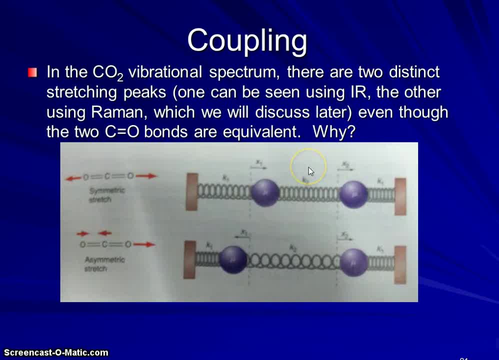 we're going to calculate this agreement that we have a ко Bond which is equal to a sẽarkan T, this her node of CO. Okay, k1, if f of in the wave relationship, then you're going to obtain a p and will over be a mod ψ, and if the power 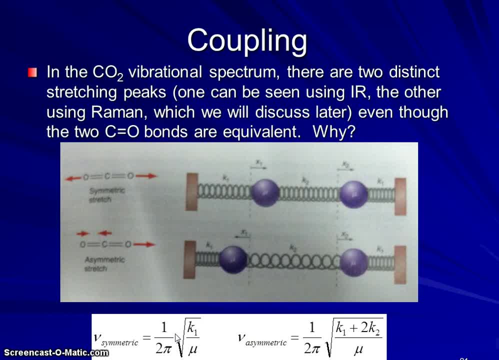 with these sensors here, Carbon is moving in between the oxygens and we would model that this way where as K2 stretches, K1 is being compressed, and as K1 stretches, K2 is being compressed, And so both of those spring constants would be factors in the overall spring constant of that vibration. 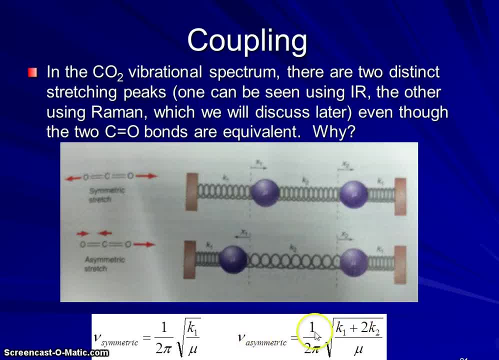 and we would calculate a different frequency using the same type of equation that we used previously. And we get this equation for handling this type of vibrational mode from physics. You probably derive that in physics- 111 or 221.. So we won't bore you with that derivation, but you can check your physics text if you are interested. 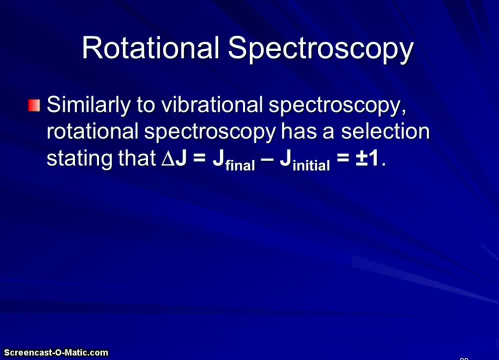 Selection rules in rotational Spectroscopy are going to be derived similarly to the way they were in vibrational spectroscopy, And what we'll notice is that we're only going to see rotational modes in our spectroscopy where the change in J, the change in level, is plus or minus 1..